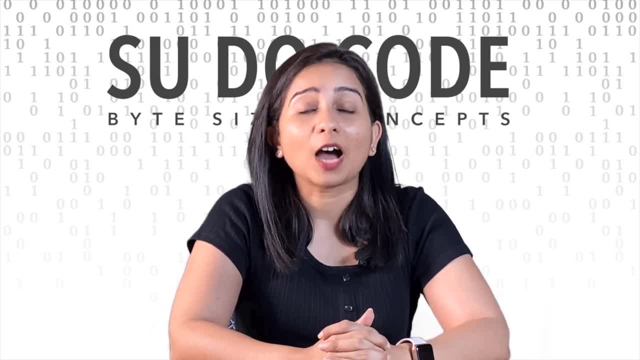 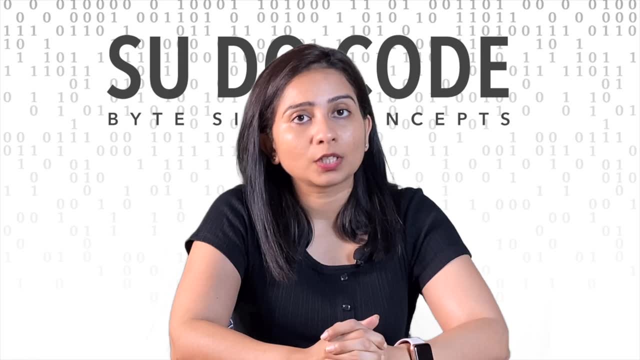 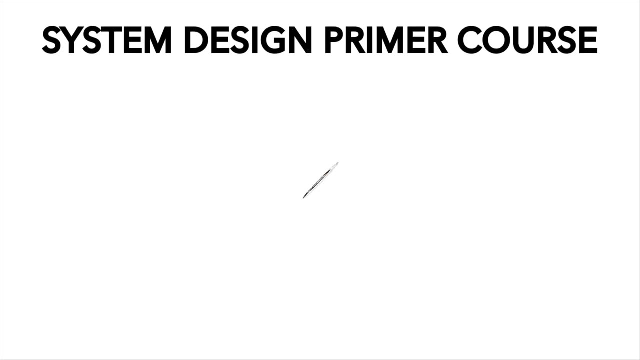 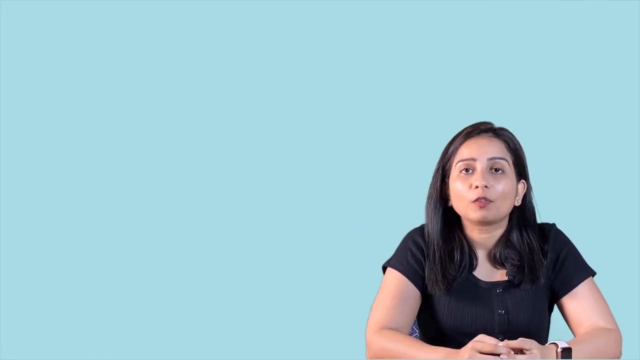 Hello and welcome to pseudocode. Today we are going to talk about how to start approaching your system design interviews. In today's video, I will discuss about what are functional and non-functional requirements and why it is important to talk about them, Since we have always talked about the building example in case of functional and non-functional. 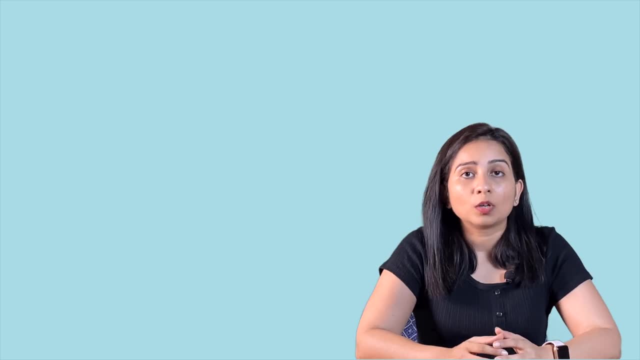 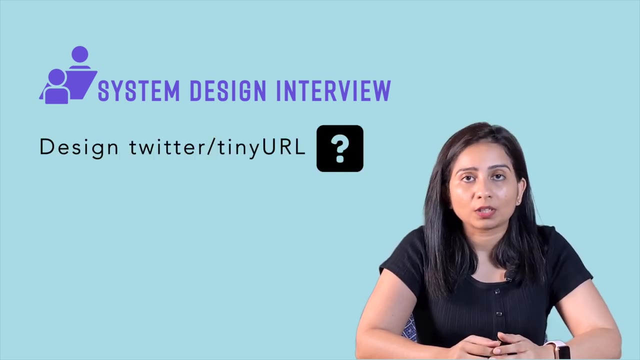 requirements as well. I will try to use the same example Now. as soon as a system design interview starts, you are given with a problem statement like design twitter or design tiny url, etc. The first step that you have to do is to try to figure out what are the functional and 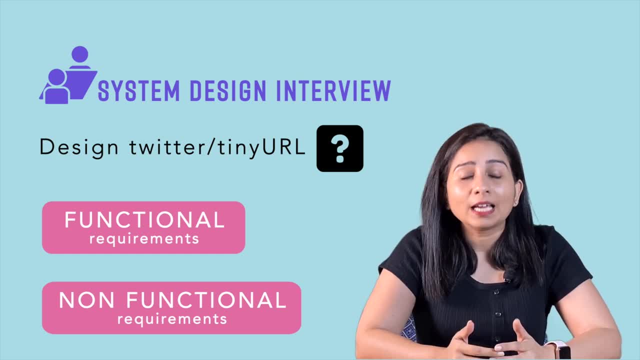 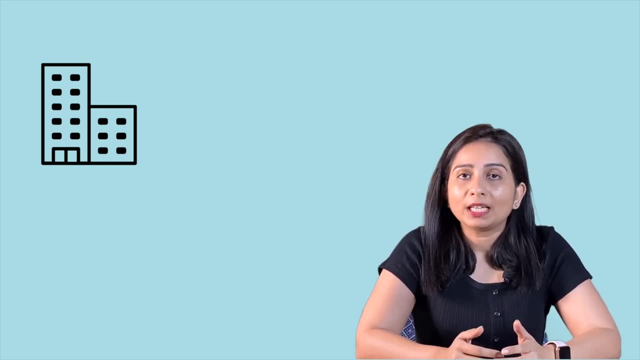 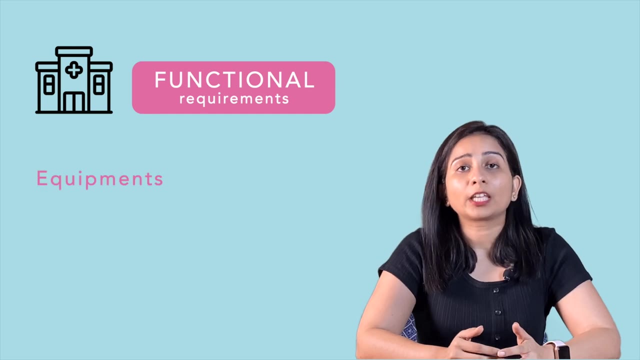 non-functional requirements. Now, before we dive in, let's see, in context of building example, what would be functional and non-functional requirements. Let's say a building has to be constructed. If that building is a building of a hospital, the functional requirements would be to have certain equipments. 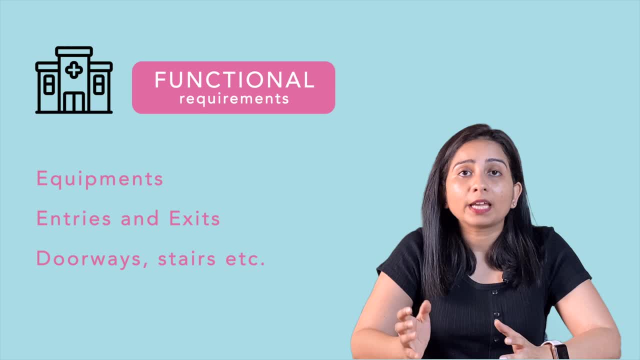 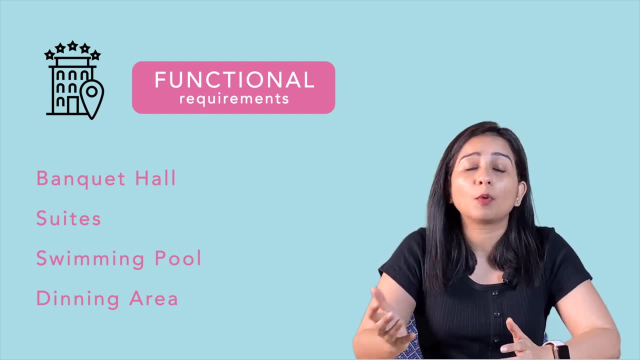 certain amount of entries and exits and the way patients can get into the building, etc. If it's a hotel, the functional requirements would be to have certain amount of rooms and certain amount of luxury available in those rooms. This is the example of functional requirements. 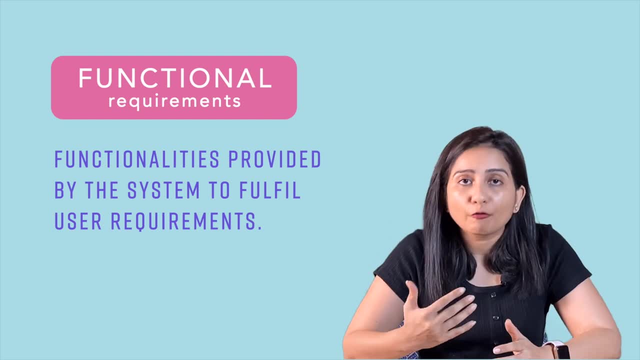 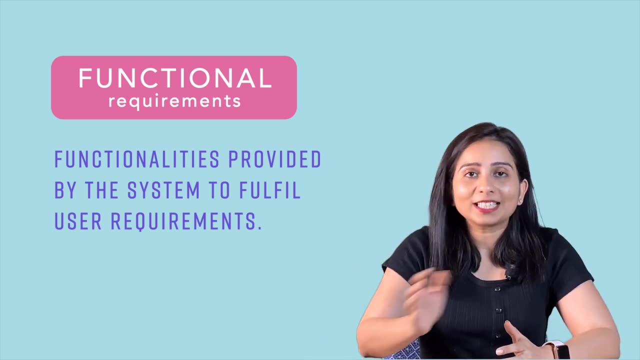 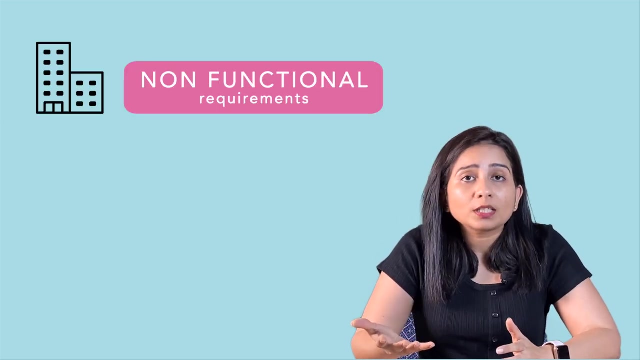 which means a system or a building, how it is supposed to function or what are the functionalities or features it is supposed to provide in order to fulfill the user requirements. So these are the functional requirements. Now, talking about non-functional requirements, the example is how many stories that building would have, or how many people that building has. 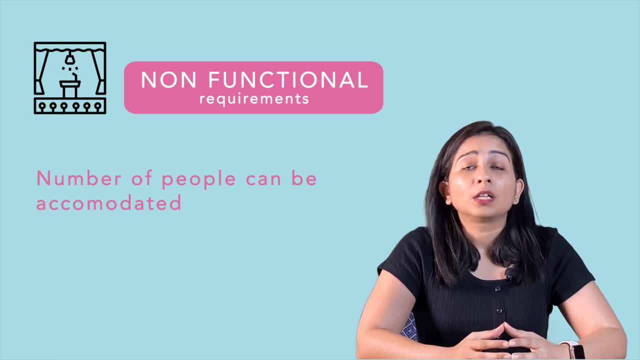 to house. For example, in case of an auditorium building, the non-functional requirement would be how many people it is supposed to see. if the sound quality of the auditorium is good enough so that the people at the back can also hear how the lightings could be placed, how many? 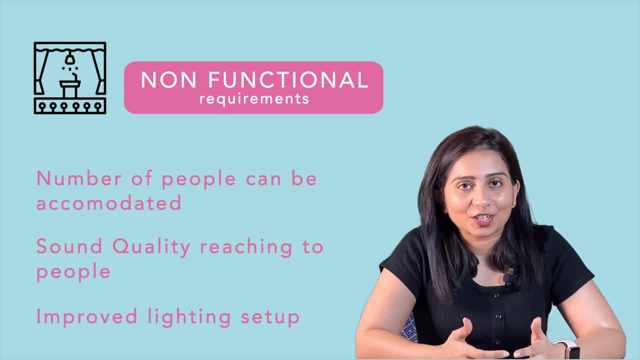 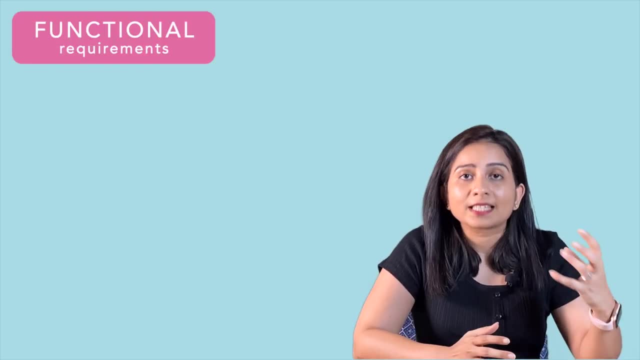 lightings could be placed, etc. This is the example of non-functional requirements. Now coming to our system design, it's very similar. Functional requirements define the system level or the component level, needs or features that users are supposed to have. If we talk about. 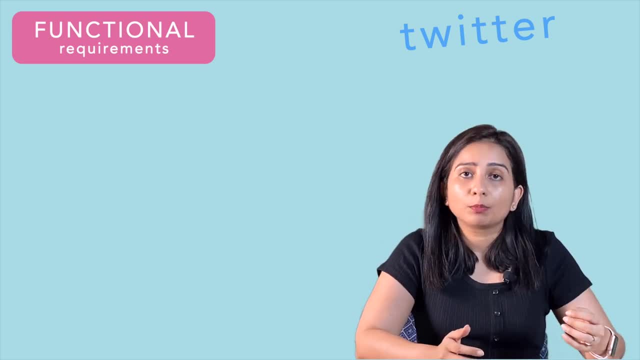 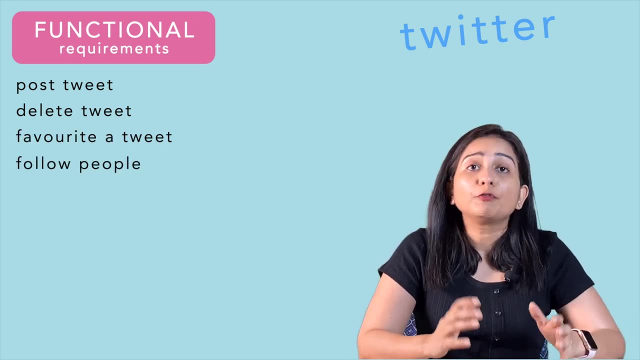 Twitter example of functional requirement is: a user should be able to post a tweet. a user should be able to delete a tweet or favorite a tweet or follow certain people, right, And if we talk about non-functional requirements, an example in case of Twitter itself would be if a person or if a user 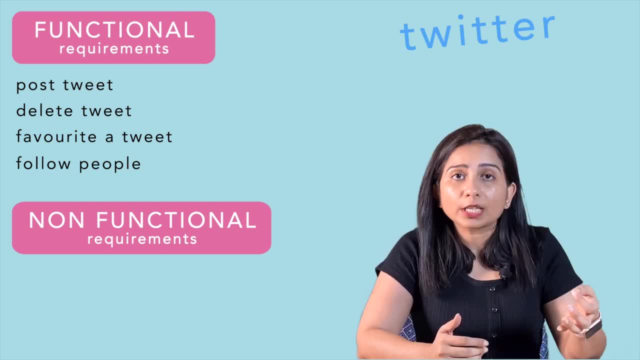 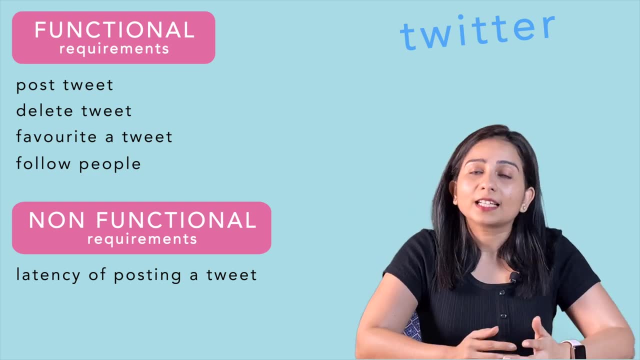 posts a tweet, it should take maybe less than a second or less than 2 seconds for that tweet to be published. In other words, we can say the latency of posting a tweet should be less than 1 second. Another example of non-functional requirement in case of Twitter example could be, let's say there: 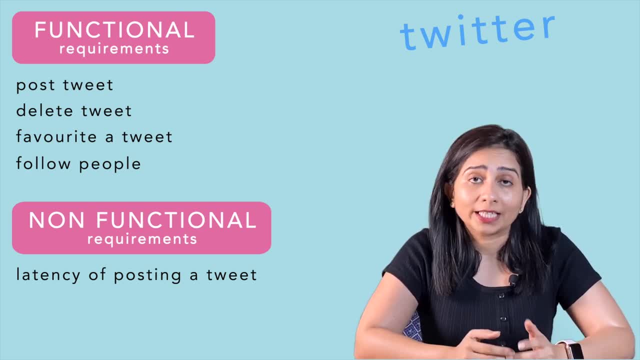 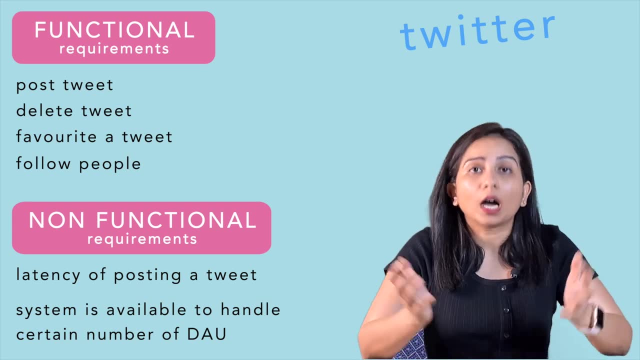 are 100 million daily active users and all those 100 million daily active users will have certain amount of transactions or requests going on and your system should be able to handle that. System should be available to handle those users right. So this is another example of non-functional. 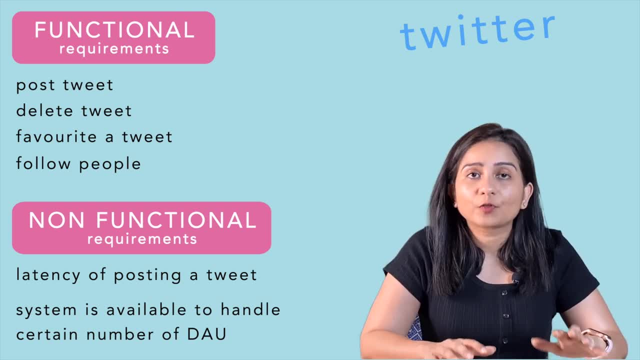 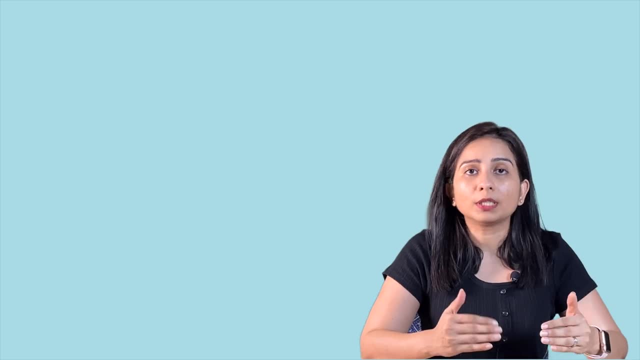 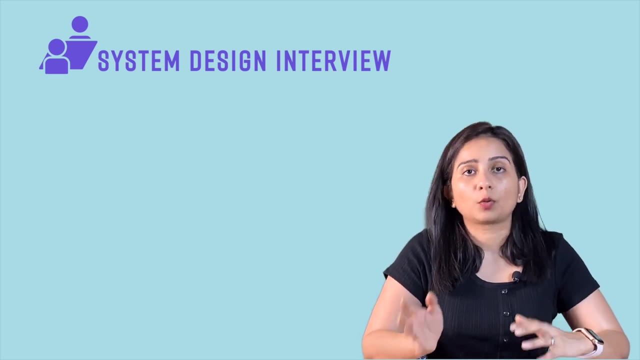 requirement in case of Twitter design. Now, if you do understand the difference between the functional requirements and non-functional requirements, now let's understand how you have to approach towards these requirements in an actual system design interview. As soon as your interview starts, put aside three to five minutes to understand these requirements Generally. 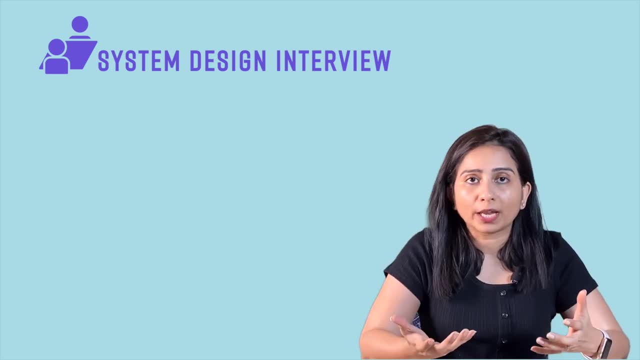 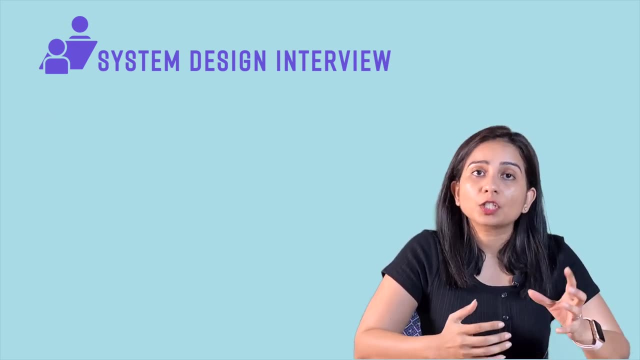 system design questions would be given to you as one-liners or two-liners, like design a ticket booking system or design an OTT platform, etc. How you have to approach these problems is: first try to dig deep inside the functional requirements. Try to understand what the system is trying to sell. 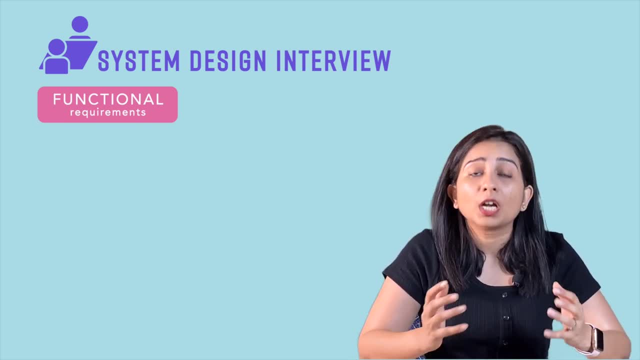 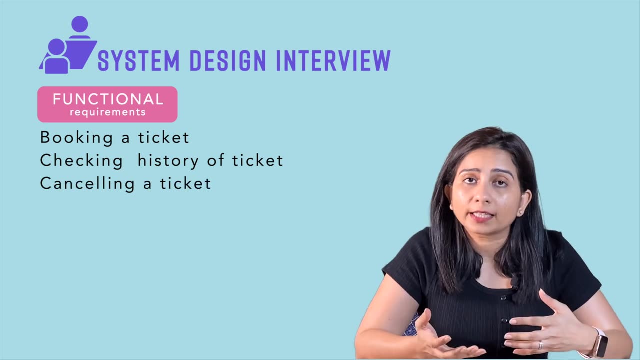 Let's say, if it's the example of a ticket booking system, try to understand what a user should be able to do apart from booking a ticket: checking a history of the ticket, cancelling the tickets, etc. Also, try to understand what other features 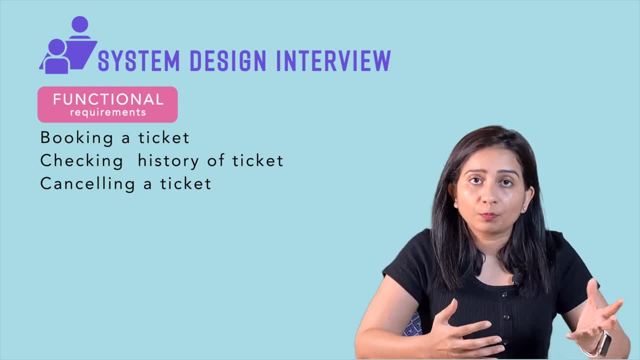 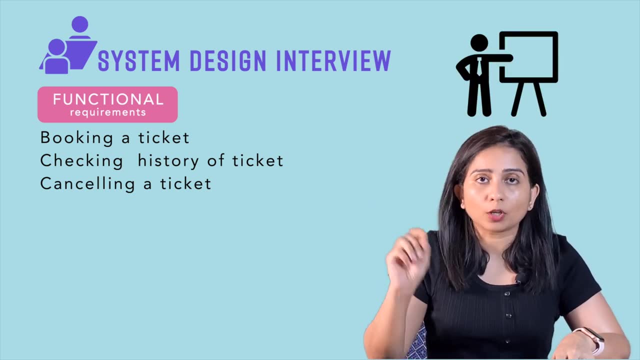 what other extended features the system is trying to fulfill. Once you get those non-functional requirements, try to make a small section on your whiteboard and keep a note down inside the functional requirements. If you do not have text on your whiteboard, try to. 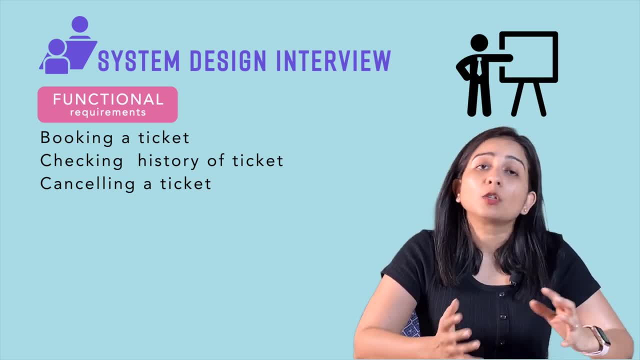 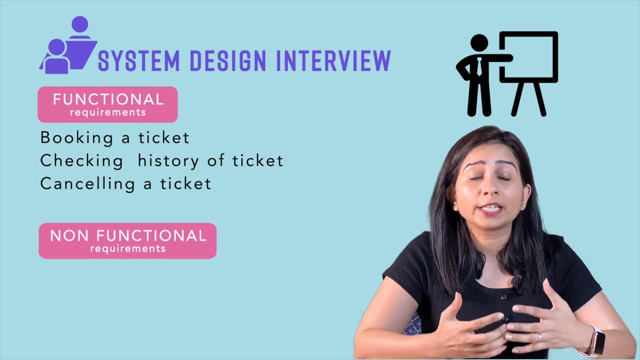 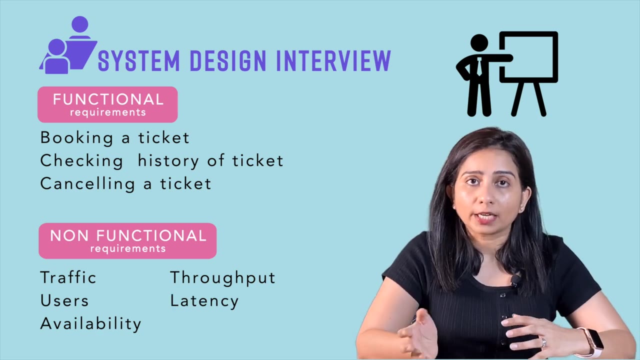 those requirements. once you do that, try to understand the non-functional requirements as well. you can ask the interviewer: what are the non-functional requirements we are looking at? uh, what do we expect into in terms of traffic, in terms of users, availability of the system, throughput of the system, latency of the system, etc. right, as you know, all these complices of 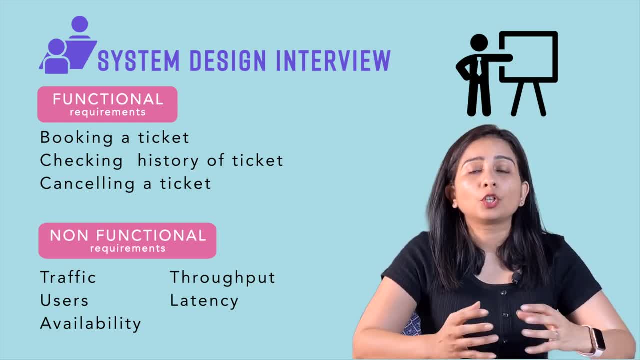 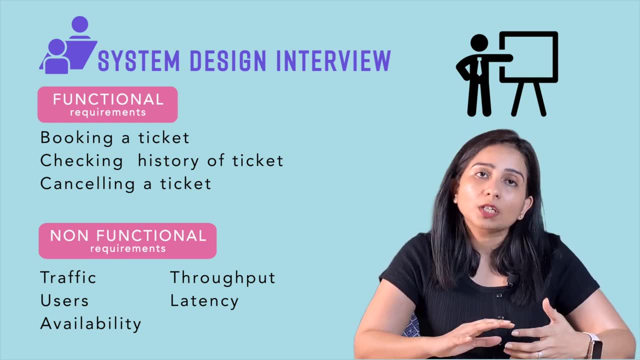 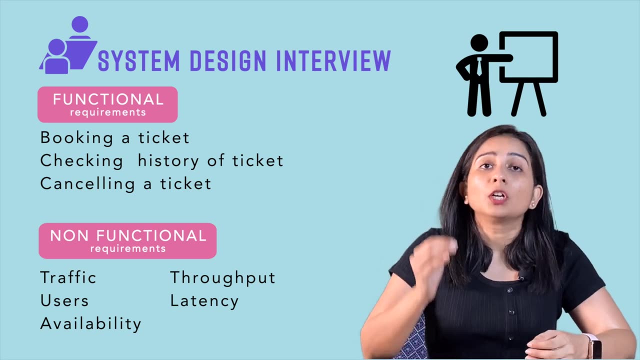 non-functional requirements. there might be cases when you are interviewing, let's say, for a startup or for a company which is not handling very large scale. in that case maybe non-functional requirements wouldn't be so emphasized on, maybe that section will be skipped altogether. but still, it is always a good idea to understand all kind of requirements. if the interviewer says: okay, we 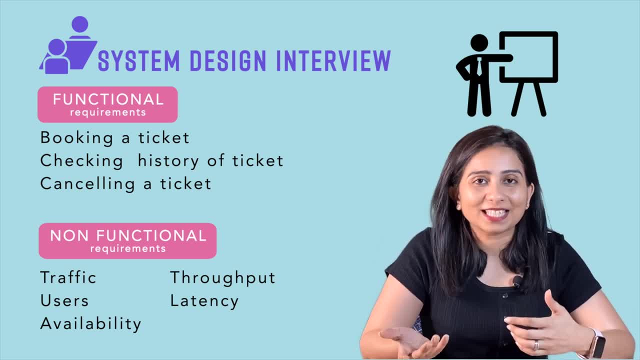 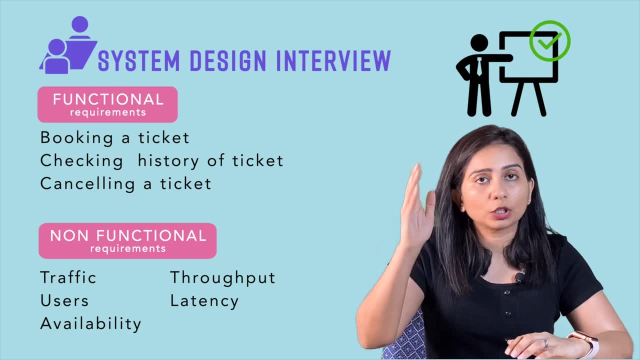 don't have to discuss non-functional requirements right now. you can just skip that section altogether. but if they do want to discuss, make sure to keep note of all the non-functional and functional requirements on the side of the whiteboard before you start actually solving the problem now. 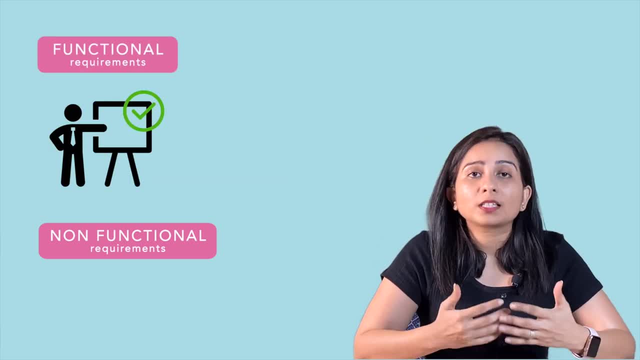 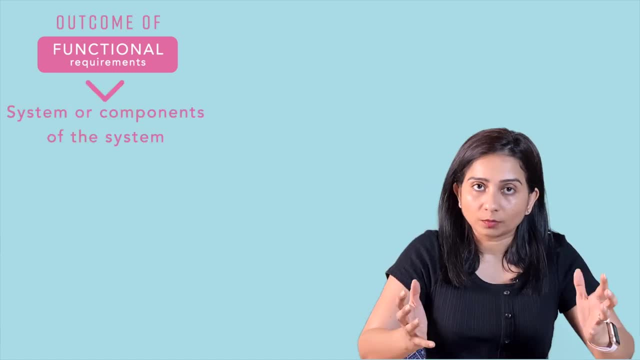 once you have both kind of requirements at your end, next step would be very natural you would understand. the outcome of all the functional requirements is generally the system or the components of the system. let's say, one of the functional requirement was to have an api, so that 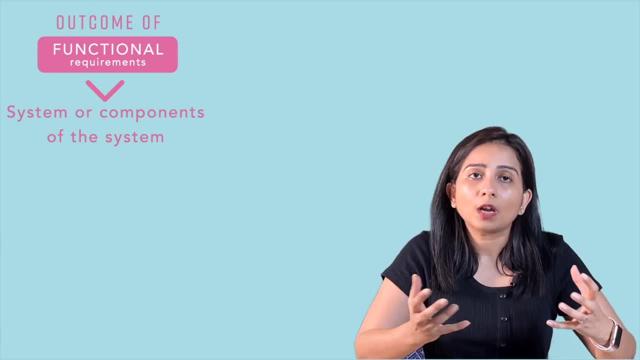 the user can book a ticket, so naturally you will understand that. okay, you have to have a set of apis which can support booking a ticket, cancelling a ticket, showing the history of tickets, etc. right, or it can be a set of some workers running a job asynchronously, or it can be two different components which 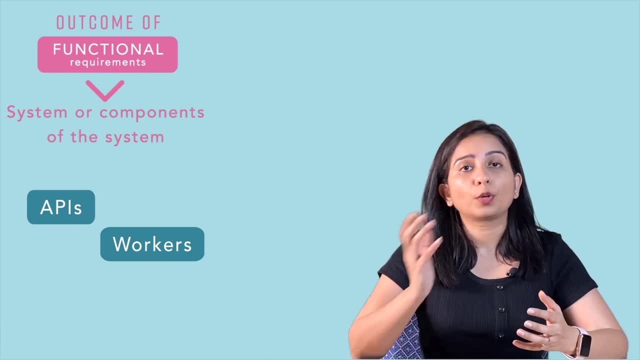 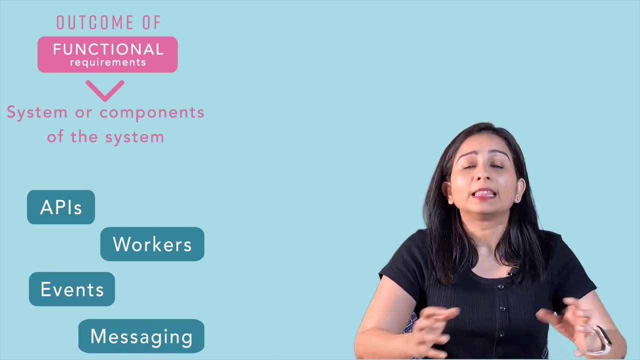 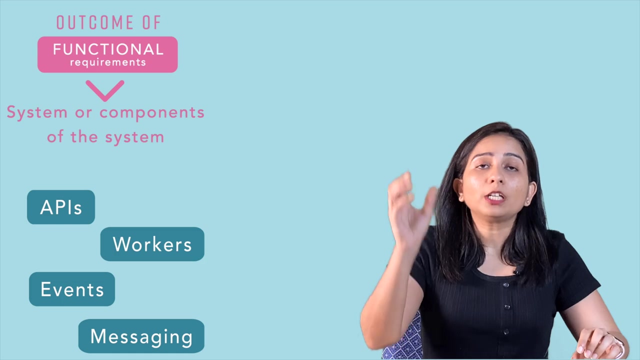 are interacting with each other, passing the information from one component to another, and that information passing is either happening through apis or events or messaging, etc. that's how you break the functional requirements and try to design components for that, distributing the responsibility of the functional requirements to those components to fulfill those. 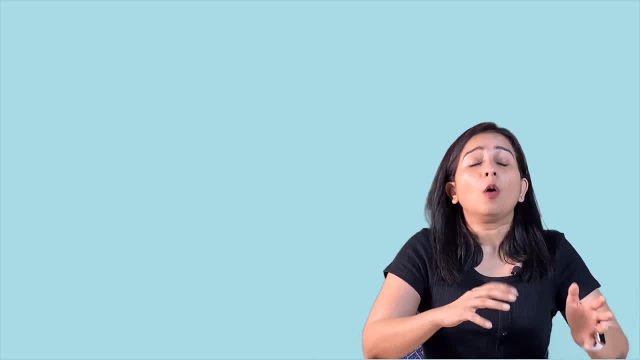 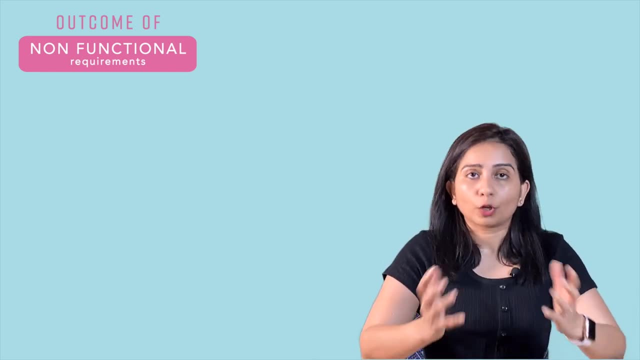 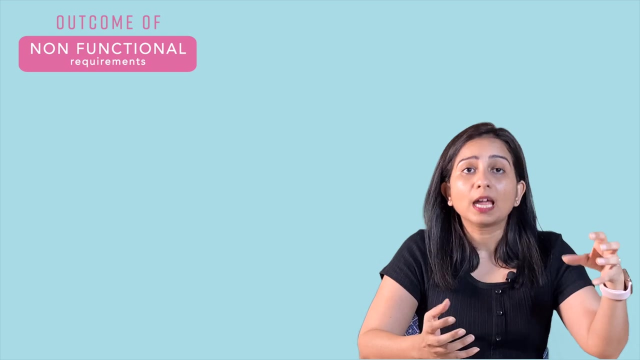 requirements now. so this is the outcome of functional requirements. when we talk about what is the outcome of non-functional requirements generally, the outcome of non-functional requirements can be one of the follows: either you try to estimate how many users or how many transactions per day have to happen, and then you try to choose resources on the basis of that. let's 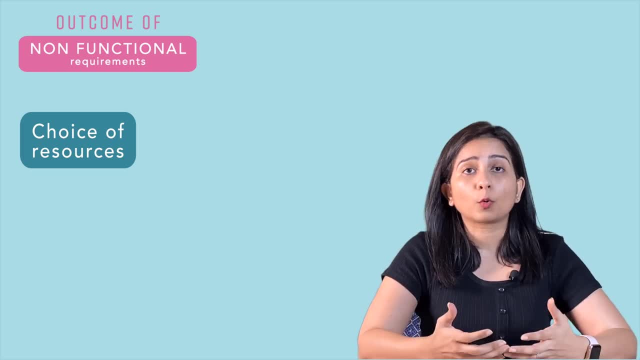 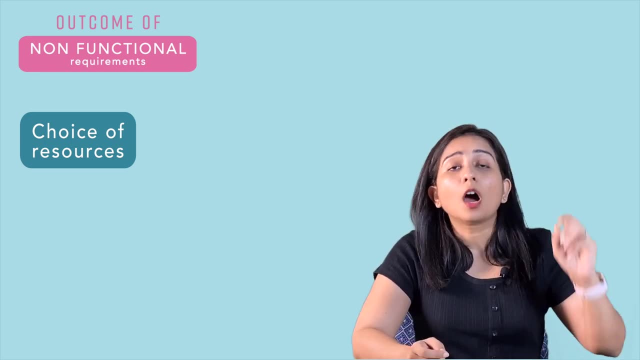 say, you have a non-functional requirement that you have to support, say one million requests per day, and you have to calculate how many servers would be needed to do so. right, so you have to find out how many requests one server can serve and then do some calculations to come up with the. 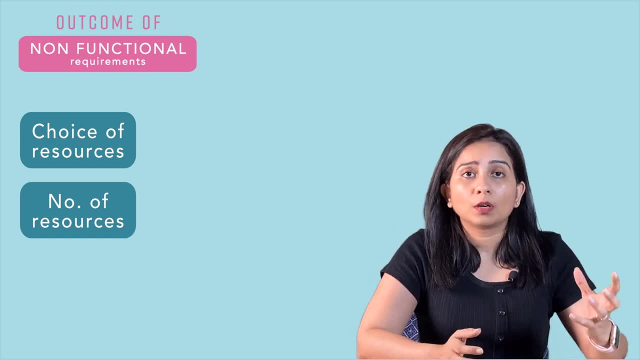 final number of servers. let's say you are trying to uh build a distributed key value storage and you want to find out the storage that is needed, and one particular technology choice is not uh serving the amount of storage that you want to have, so you have to go with another tech stack. 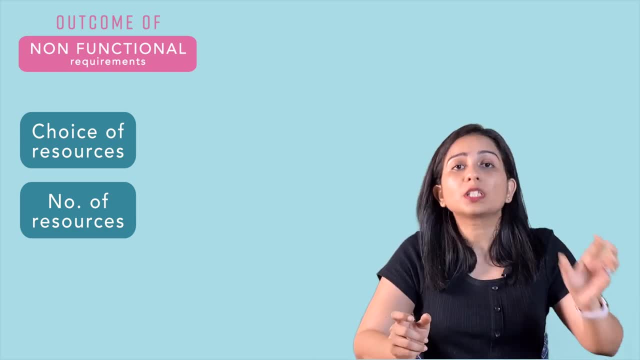 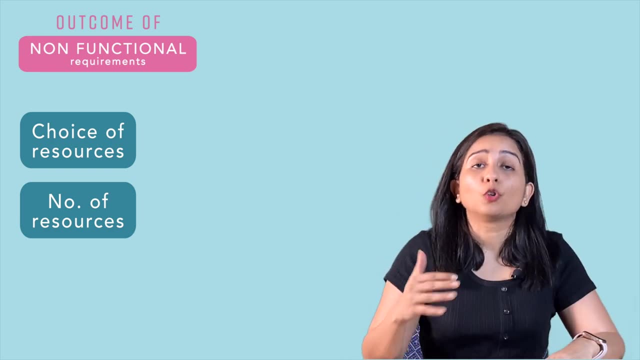 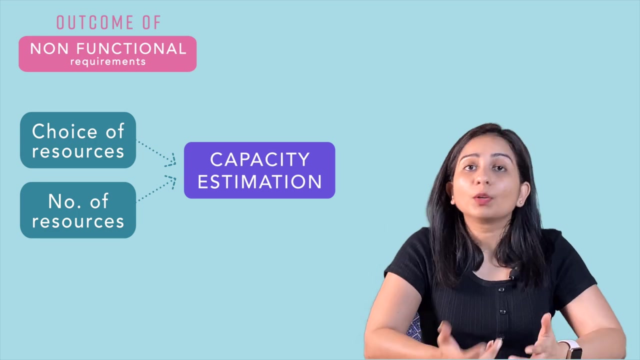 and using these requirements, using these calculations, you can actually support your choice that, because we have such huge data to store, i would like to go with this tech instead of this. so non-functional requirements through capacity estimation can help you make these decisions of different tech choices right. one more example is suppose one non-functional requirement says: 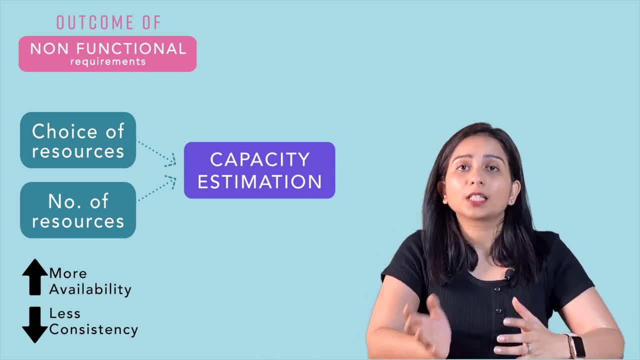 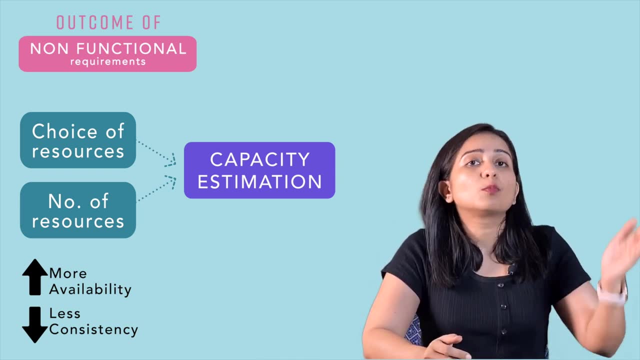 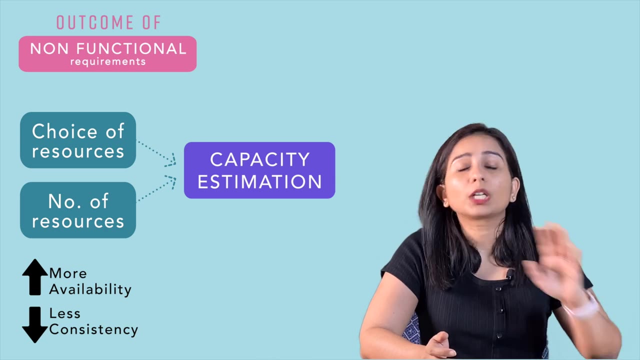 that the system needs to be more highly available rather than consistent. if that happens, and if you remember the cap theorem video, you can quickly conclude that if availability is more important than consistency, then you have a choice to pick from so many no sql data stores rather than going with a sql data store given another other use cases and 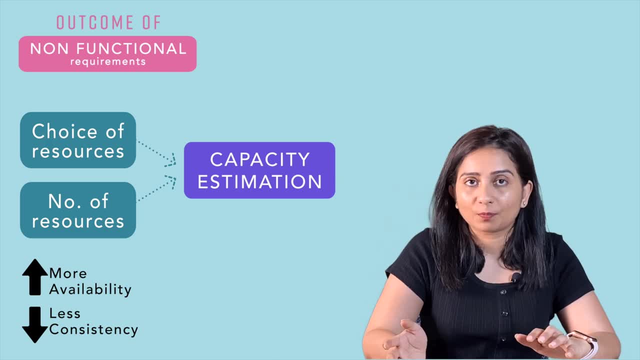 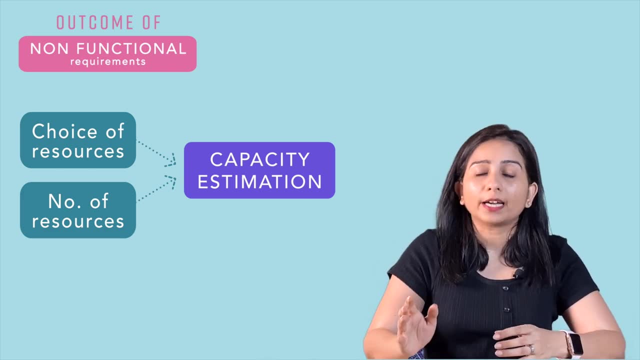 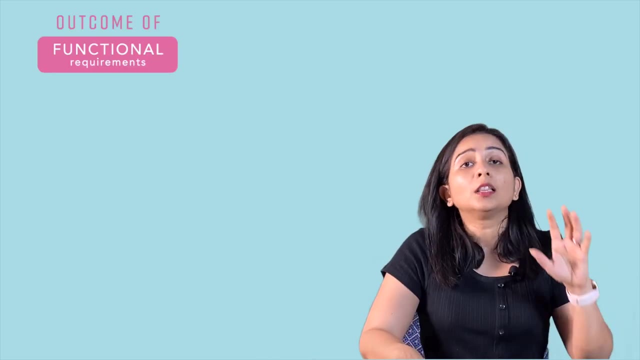 requirements are also fulfilled by that particular no sql data store. so these are the choices or decision making steps that can actually help you once you understand the requirements and you can bifurcate the requirements into functional and non-functional. just to summarize again, the outcome of functional requirements would be your system design diagram, your component and architecture. 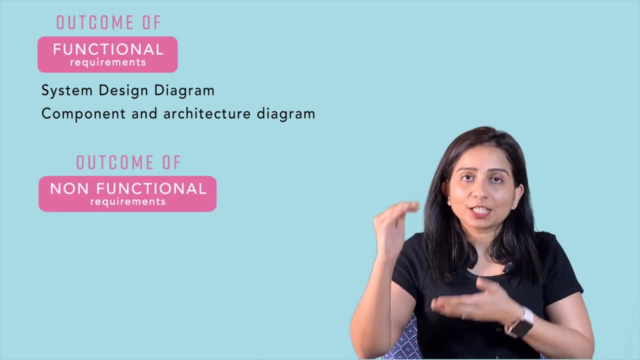 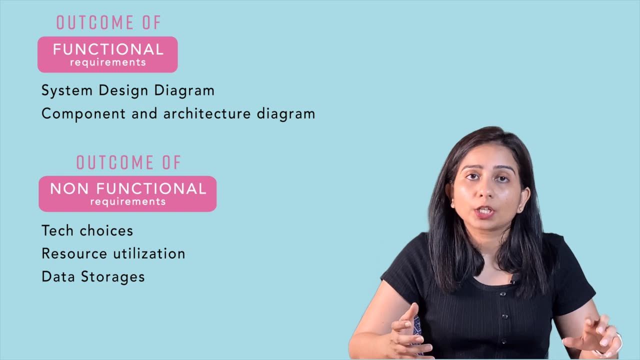 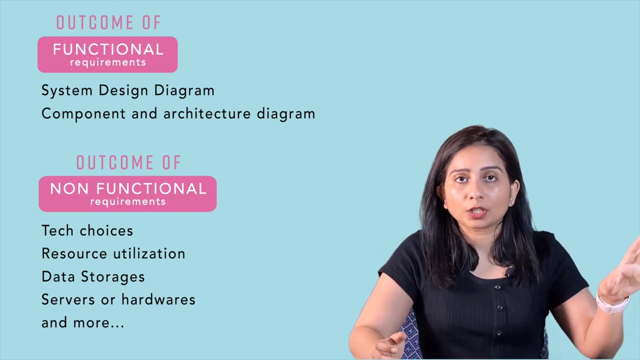 diagram. the outcome of non-functional requirements, after a series of capacity estimation and calculation steps, would be certain tech choices, certain resources, what kind of data storage? what is the? what kind of servers or hardware or different resources that you would need to fulfill that architecture diagram on which the whole system is going to function. on last but, 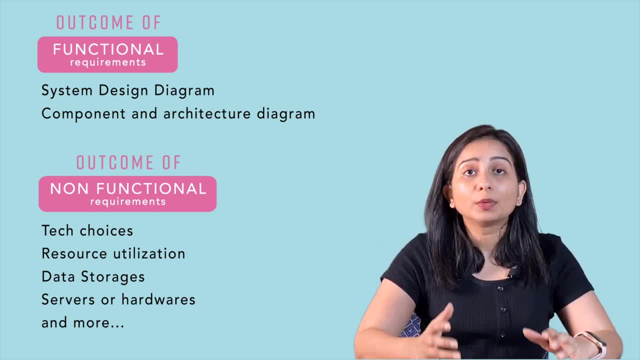 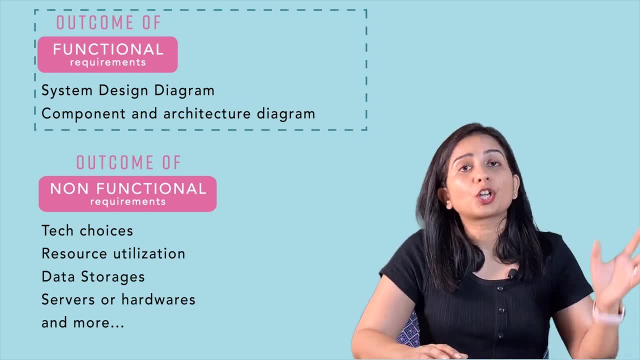 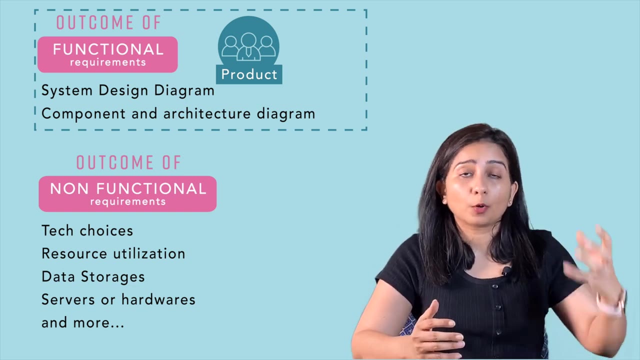 not the least, when you do actually go into the real world and build real world systems, when you get a job and you join a company and you actually work on these systems. functional requirements are something which come from a product or user perspective or business perspective, where business needs certain features to be developed or a product manager needs certain features to 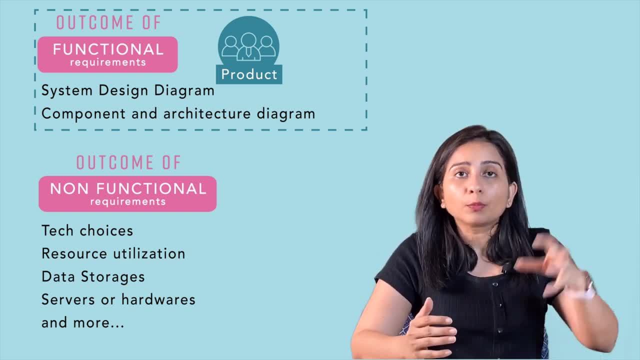 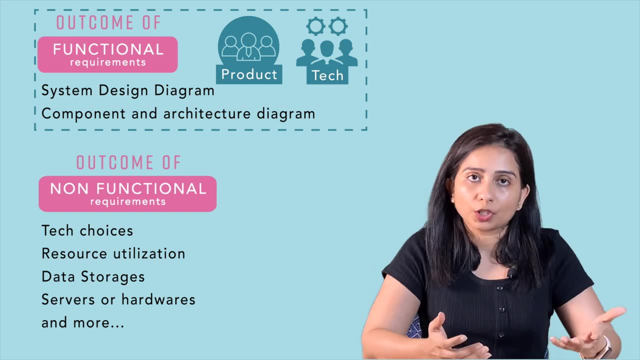 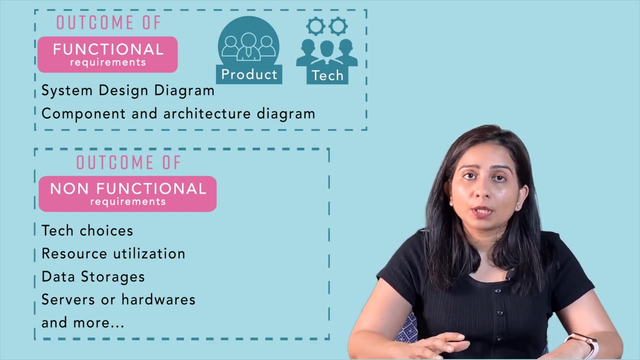 be developed that can be experimented on. those will be your input for functional requirements. tech teams which need certain features in order to fulfill their task can also be the input for your functional requirements, but generally these are the people who will come to you with functional requirements. on the other hand, non-functional requirements would be part of more engineering.